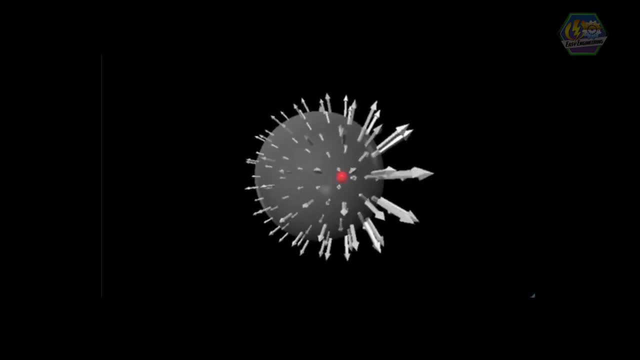 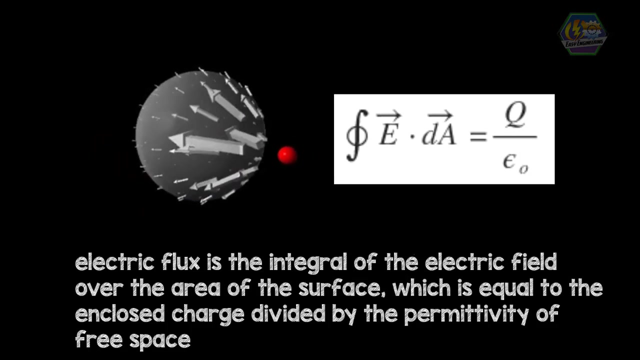 A closed surface, in this case is just a surface of any shape that completely encloses a charge, like a sphere or any other three-dimensional shape. Mathematically, this equation says that electric flux is the integral of the electric field over the area of the surface which is: 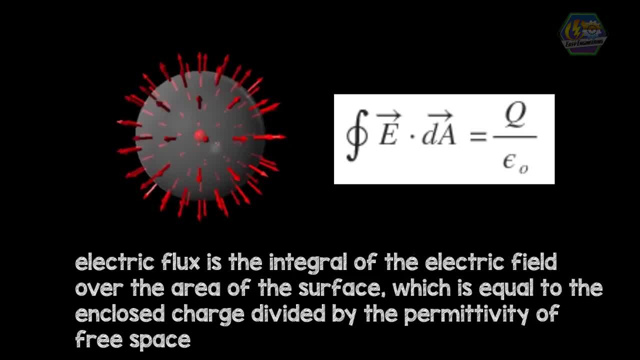 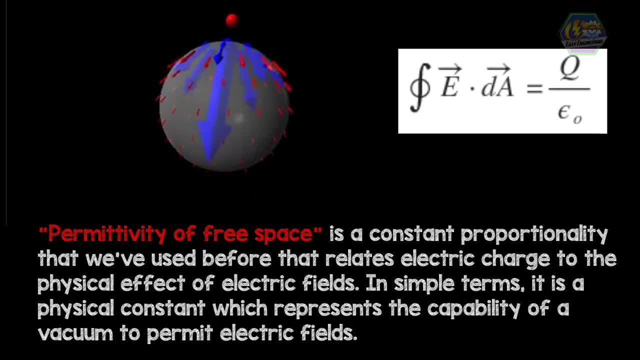 equal to the enclosed charge divided by the permittivity of free space. The permittivity of free space is a constant proportionality that we've used before that relates electric charge to the physical effect of electric fields. In simple terms, it is a physical constant which represents. 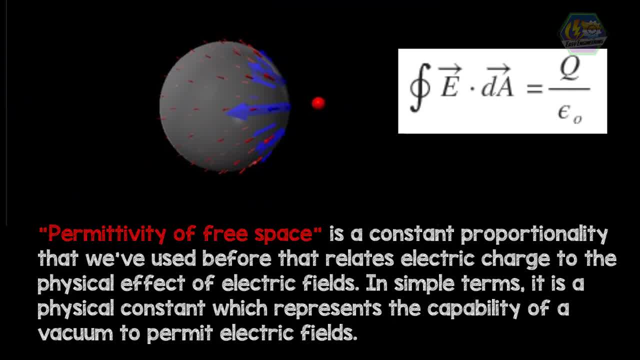 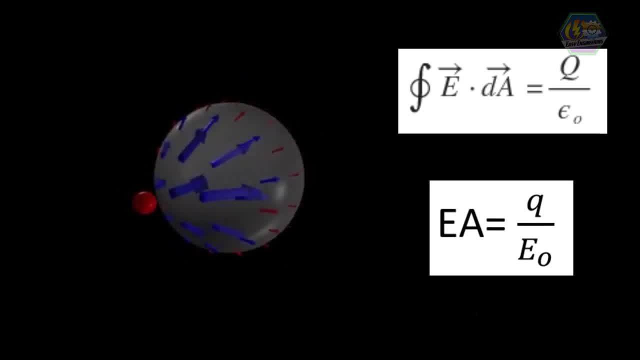 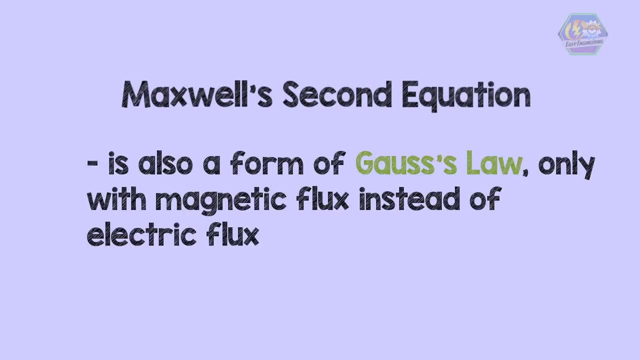 the capability of a vacuum to permit electric fields. If the electric field is constant over the surface, then the left side of the equation becomes E times A. Now let's proceed to the second equation. Maxwell's second equation is also a form of Gauss law, only with magnetic flux instead of. 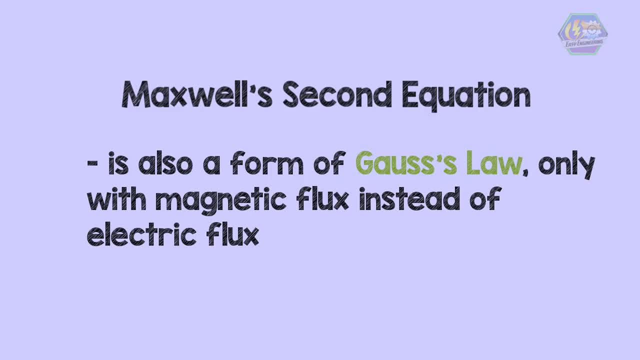 electric flux. As a result, the electric flux through a closed surface is proportional to the magnetic flux. The magnetic flux through a closed surface is proportional to the magnetic flux. As we've discussed before, magnetic sources are always dipoles, which means it has a north and 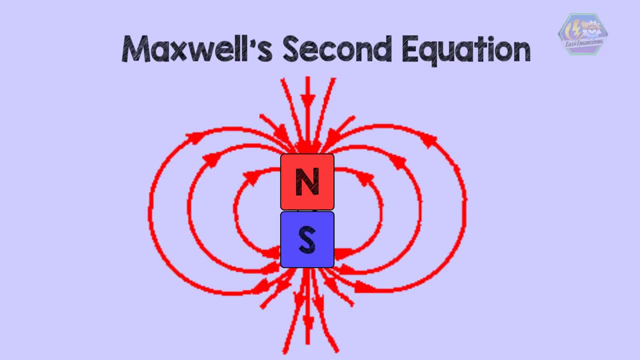 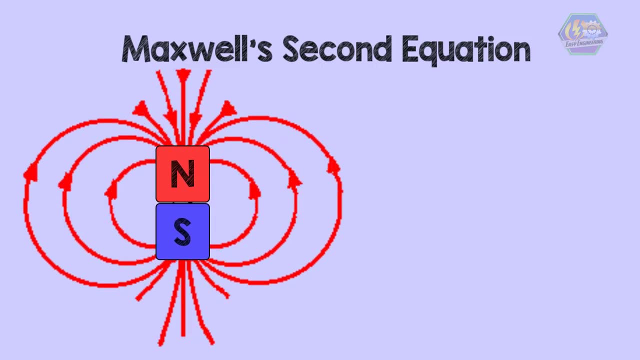 south pole and the magnetic field lines leave from the north pole and return back to the south. When you're looking at how a magnetic field interacts with the surrounding surface, you see that the field lines that leave the surface out of the north pole must enter back. 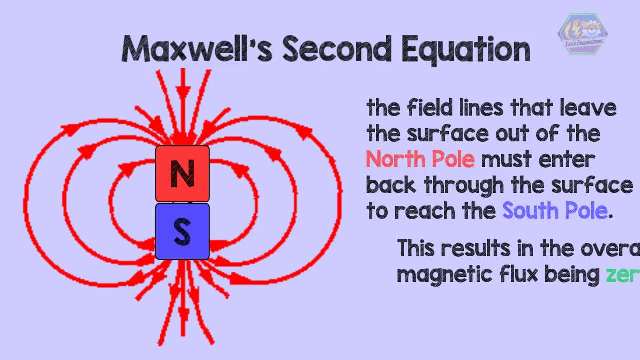 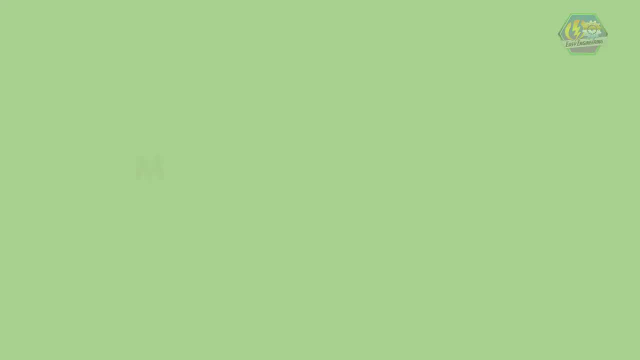 through the surface to reach the south pole. This results in the overall magnetic flux being zero. Now let's move onto the third equation. Maxwell's third equation doesn't have anything to do with Gauss law. Instead, it's Faraday law. As you can recall, Faraday's law of induction says that a changing magnetic 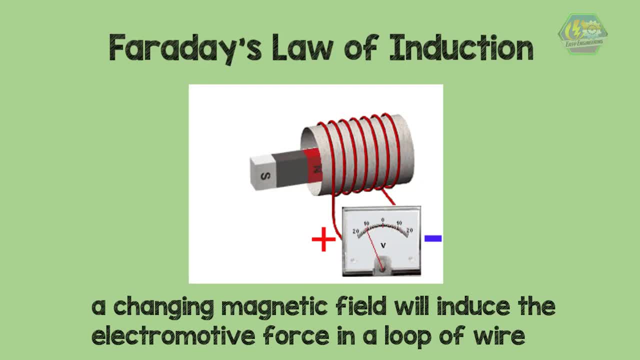 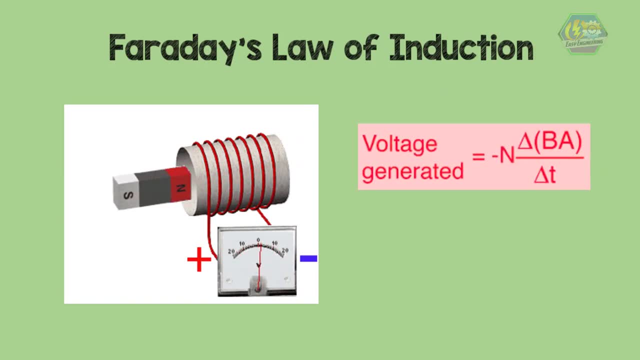 field will induce the electromotive force in a loop of wire. Maxwell's version is a more general simplifying Faraday's law to show the value of that induced emf. And that's how you predict that an now sinful orosters the maximum magnetic force from an electricody approach. 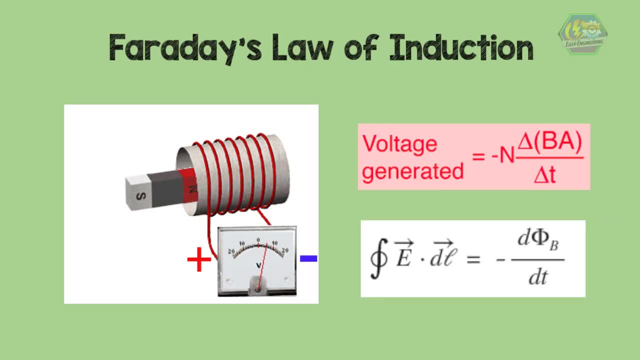 That's all we'll talk about in this video. says that EMF is equal to the line integral of the electric field over a closed loop. So with this equation you can see the connection between a changing magnetic flux and an induced electric field. Maxwell's first and second equations were so similar, one for electric